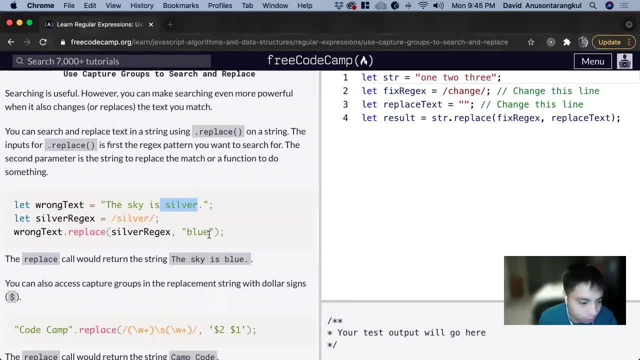 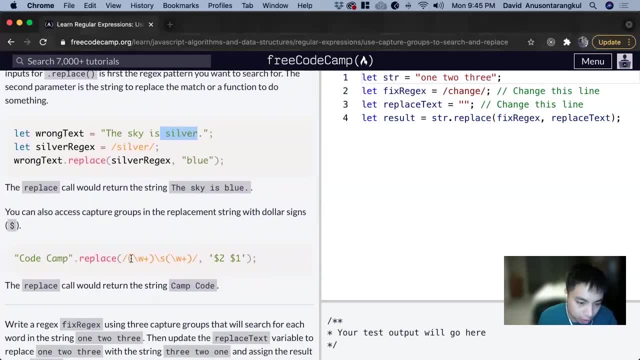 we're going to look at the silver inside of the string and replace it with blue, and then we can also use capture groups to access it. so if you're not sure exactly what the exact word, but know it's going to be a word, and then. so here we have the first word and then the second word, and it's. 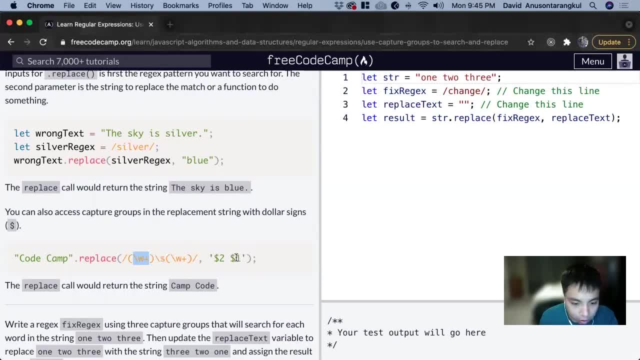 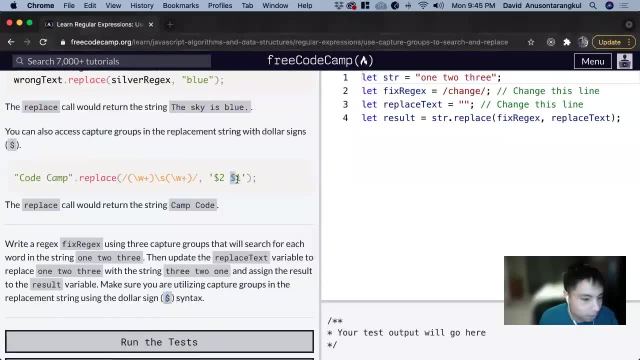 separated by a space, so this is associated with one, and you need to use the- the dollar sign, I believe- to access the capture group. so we're going to replace it with the second one going first and then the first one going afterwards, so CodeCamp will be camp code. 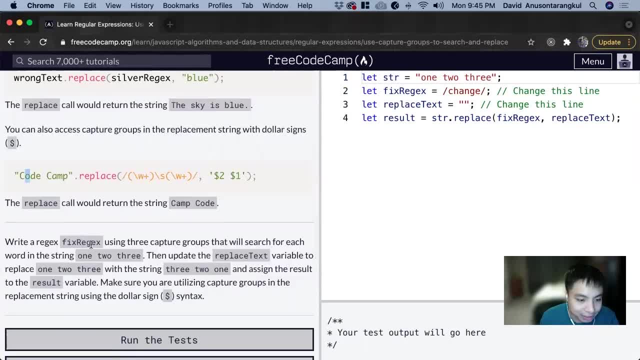 So for this example, we want to write the regex fix regex using three capture groups that will search for each word in the string one, two, three, then update the replace text variable to replace one, two, three with the string three, two, one and assign the regex to the string three, two, one. 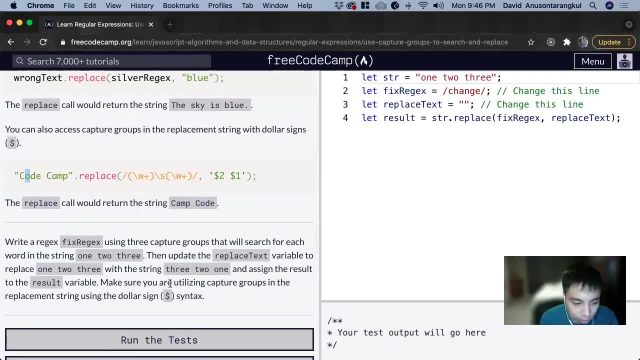 Then the result to the result variable. make sure you are utilizing capture groups in the replacement string using the dollar sign syntax. so we have here and now let's create this part of it. so we know that we're gonna. we have to create capture groups, so the first one be parentheses, slash w for any alphanumeric word character. 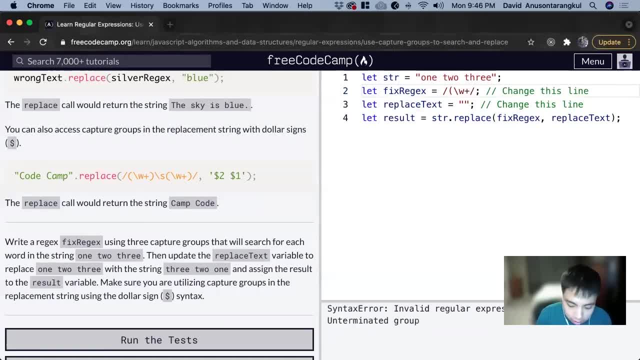 and then we do plus. that occurs at least once, and now we close it. and now we have a space by a variable. and now we have it again for the second word, space by a variable, let's say space by a space. and now we have it one more time. 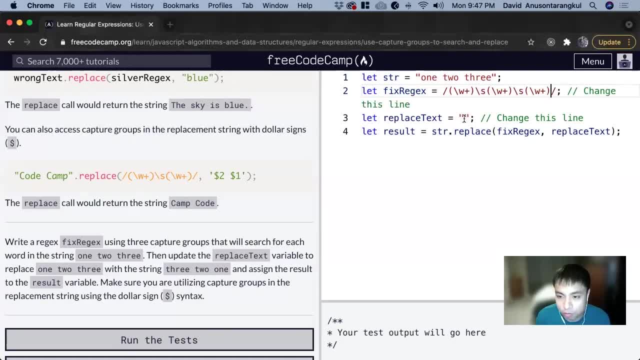 great. so now let's replace it. so we're going to change the order of it. so instead of one, two, three, we want three two one. so this is one, this is two and this is the third capture group. so we want to put the third capture group first, and then the second one, and then the first, and now we can see it in the 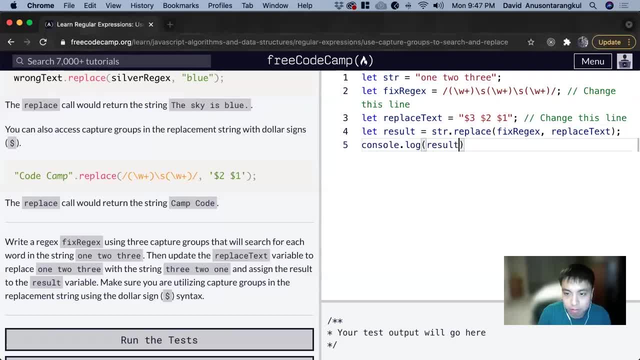 console log that one, two, three becomes three, two, one. and that's it for this one. thank you so much.